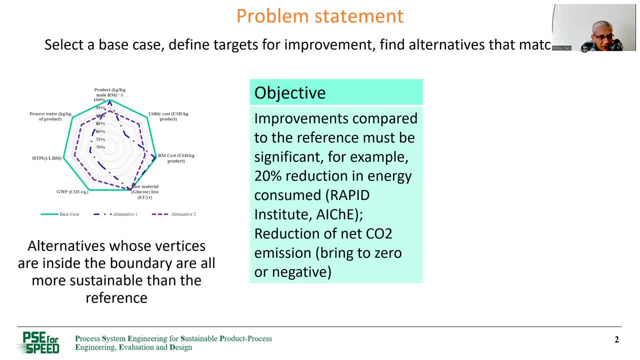 The objective is to find alternatives for which at least two of those vertices are significantly better, and all the others can be the same as the base case, but never crossing the green boundary. The means to achieve these alternatives: there are different ways to get them. 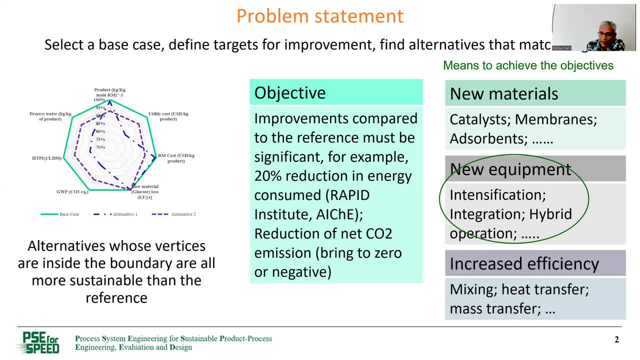 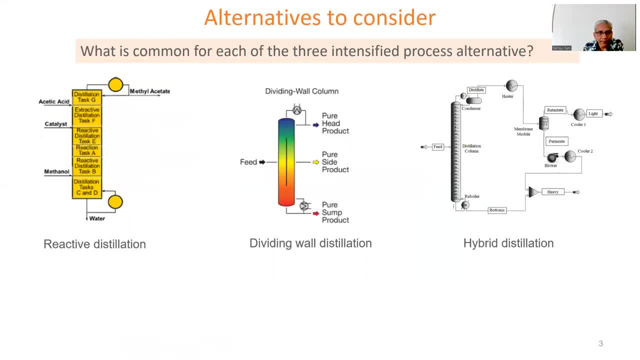 What we are concentrating on in this presentation are new equipment, that is, intensified equipment, integration or hybrid operation. The three intensified operations we are going to consider are reactive distillation, dividing wall column or hybrid distillation. What is common in each of the three intensified 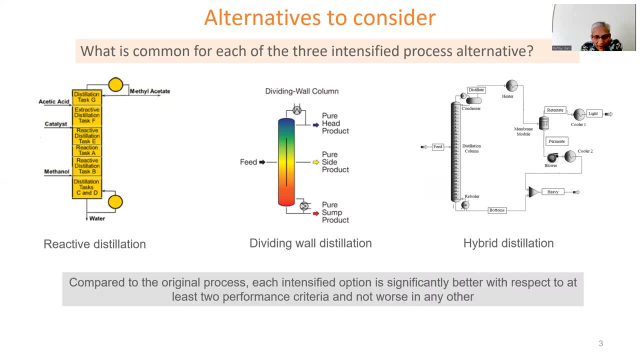 process alternatives. Compared to the original process, each intensified option is slightly or significantly different from the original process. Each intensified option is slightly, significantly better than with respect to at least two performance criteria that we discussed in the previous slide, and not worse in any other. 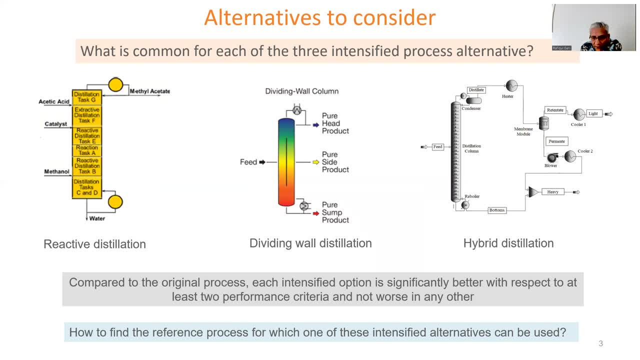 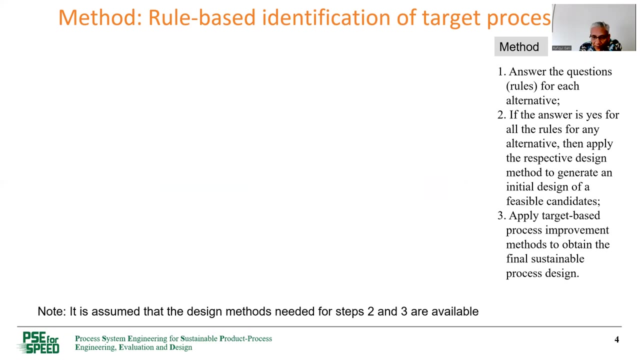 And the issue is how to find the reference process for which one of these three intensified alternatives can be used. So which is the process where they can be applied? The method is very simple. We have three steps. The first step: we apply a set of rules to find the answers. 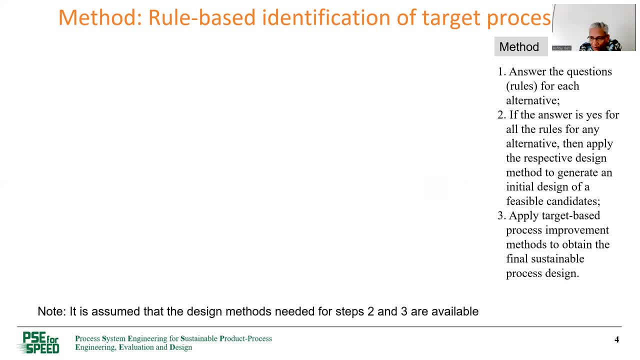 If the answers are yes, then we use in step two the basic design to design the alternative and in step three we analyze and use some targets to improve the design And we assume that the design methods for step two and three are available. 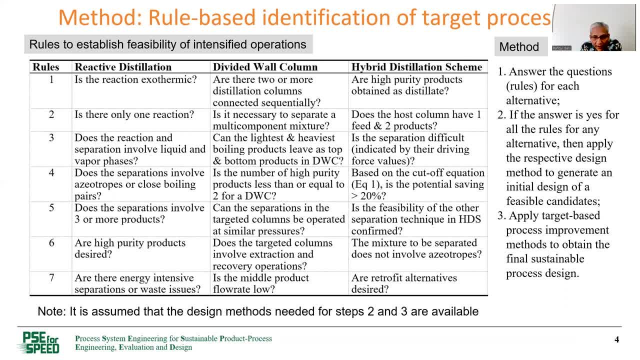 So what are the rules In each case? there are three steps, There are seven rules, or in other way, we can put seven questions for each type of intensified operation and the answer needs to be yes for each of those. If the answer is yes, then it means one of the three types can be applied. 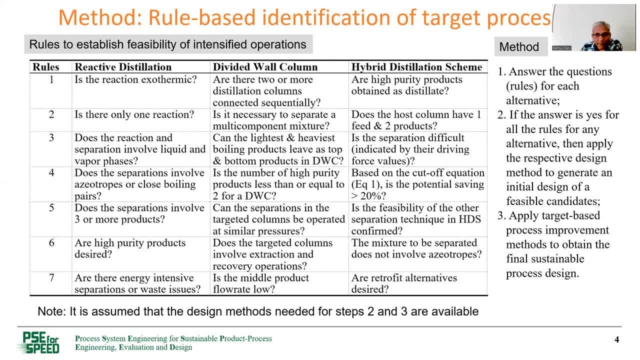 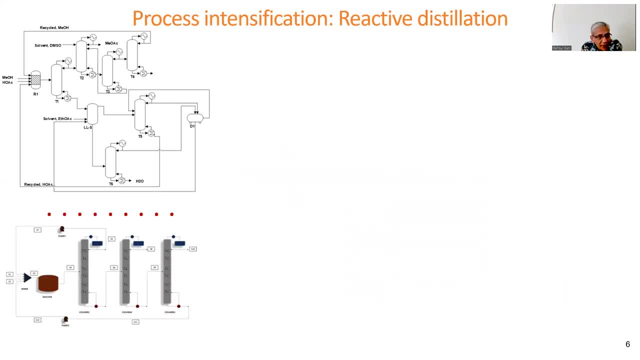 And then we apply steps two and three. I will go through the questions and the answers with the examples Of each case. So let's take the first case: reactive distillation. Reactive distillation commonly chemical processes where there is a reactor, followed by separations. 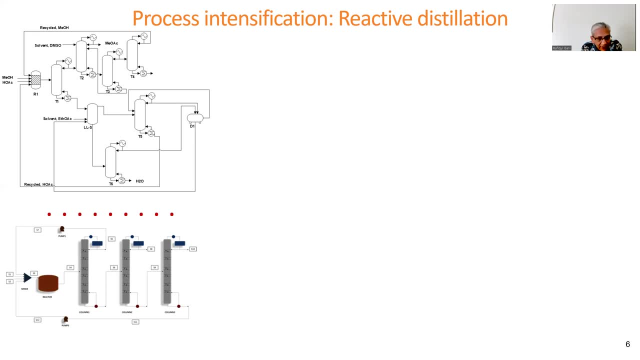 Usually distillations. these kind of processes that you see on the left can be converted into a reactive distillation. So let's look at the seven questions and answers. So is the reaction OK? OK, that is taking place. exothermic: 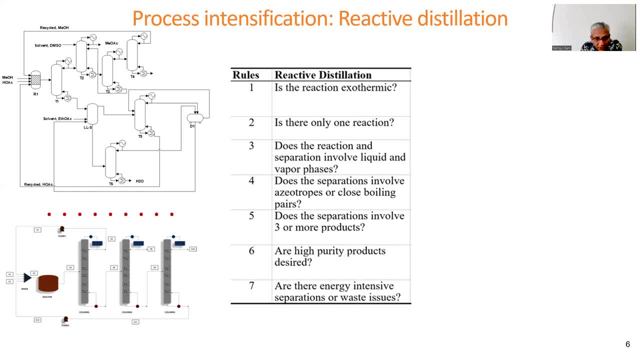 Yes, it needs to be exothermic so it will generate vapor. Is there only one reaction? Yes, but if there is more than one, it can also be handled. Does the reaction and separation involve liquid and vapor phases? It needs to be yes, so we have liquid and vapor phases. 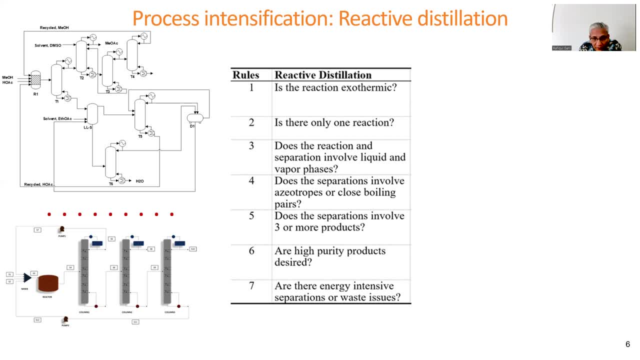 in the reactive distillation. Does the separations involve isotropes or close boiling pairs? Yes, because then the incentive to use reactive distillation would be there. Does the separations involve three or more products? Yes, then we can do the separations and see what happens. 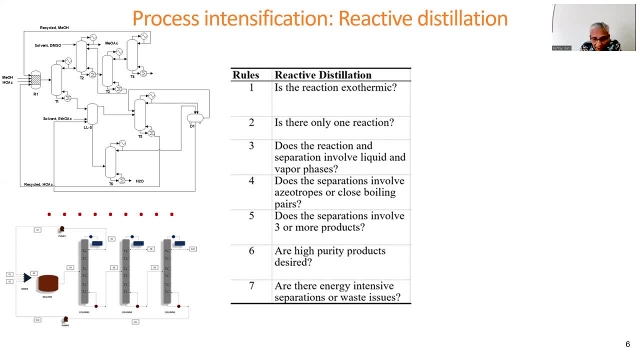 But if there are more than two products coming out of the system, then extra separation may be needed. Are high purity products desired? Yes, there's the incentive to use reactive distillation. Are there energy, energy intensive separations or waste tissues? 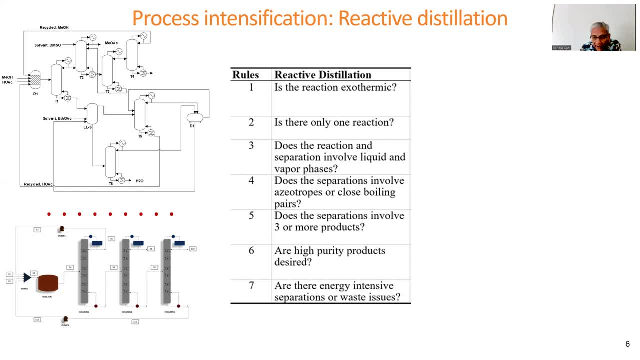 Yes, then there is the incentive to use reactive distillation. Then, if answers are yes, all the answers are yes, We have a reactive distillation and the questions that you see are the design answers. That is, what is the condenser duty? 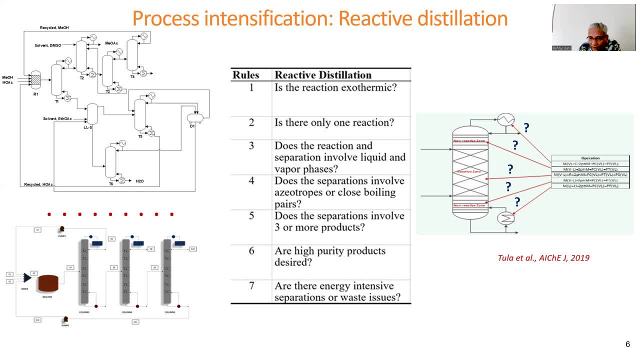 How many stages are needed for the nonreactive stages above the reactive zone, How many stages are needed for the reactive zone, How many stages are needed below the reactive zone for the non-reactive stages, and what is the revolver duty? If we answer all these questions and find values for them- and it's a feasible- 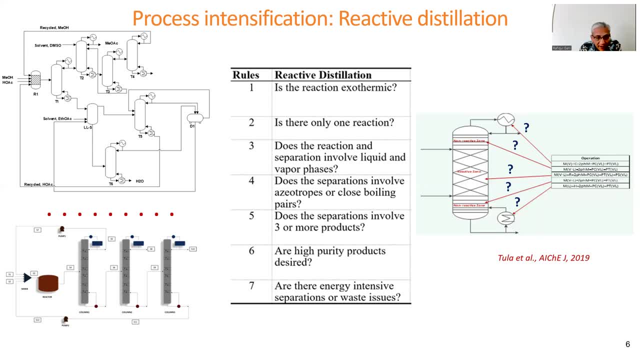 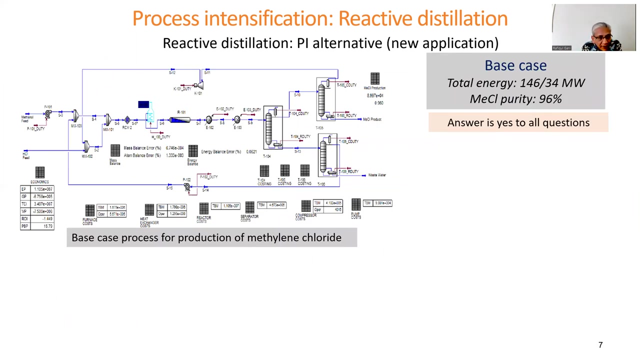 reactive distillation design. by definition, it will be better than the original process. So what we are looking for is, then: which is the process which satisfies these seven answers, and then to verify that the reactive distillation is, in fact, better. Here is a new example that we have not published before. We have methylene chloride production. 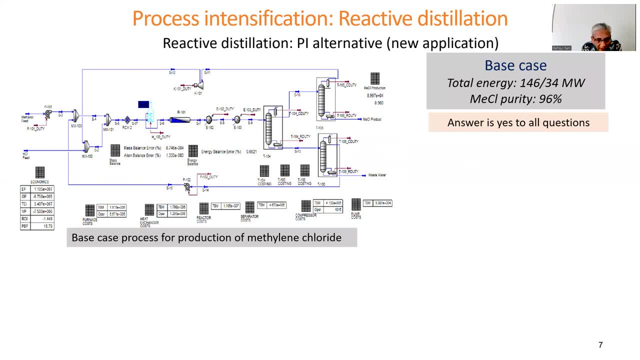 from methanol and hydrochloric acid. All the details of the process can be found in the literature. We have taken this details and performed the simulation and matched the design. You can see that the flow sheet has been reduced to a reactive distillation. and since all the answers 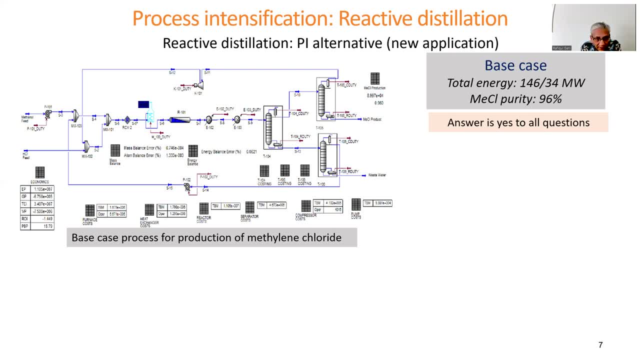 are yes to the seven questions. we know that a reactive distillation, if it can be configured, will be significantly better. So the reactive distillation design consists of two parts: First, reduction of this flow sheet to a reactive distillation configuration and then designing the reactive distillation. 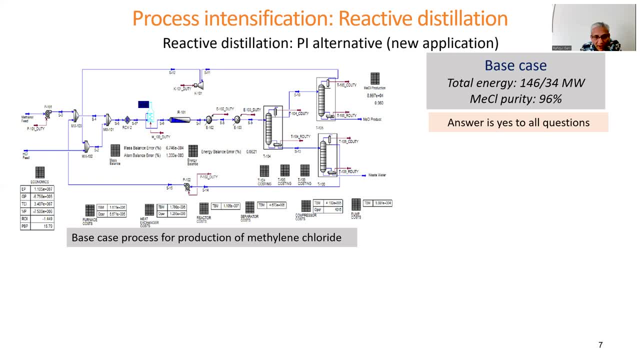 Unit operations can be combined through the phenomena that are occurring and they need to be adjacent to each other, So the reactor, followed by the first distillation column, can be combined. Once they are combined, then the second distillation column can be combined and then the third. But if there are two products coming out of the third, 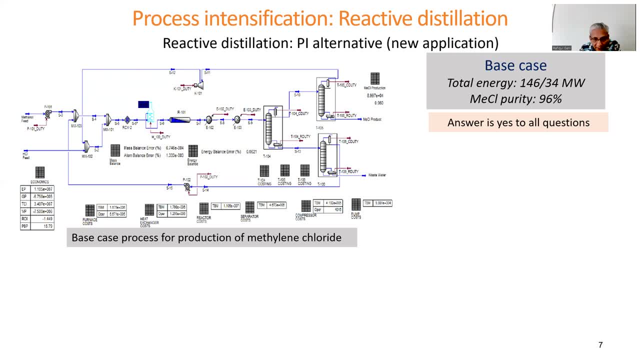 then we may need to keep that separate, because one reactive distillation will have two products. So based on this we design the reactive distillation column and the third distillation column is a separation unit, a distillation, And we can see already from the results of this that the reboiler duty for the reactive 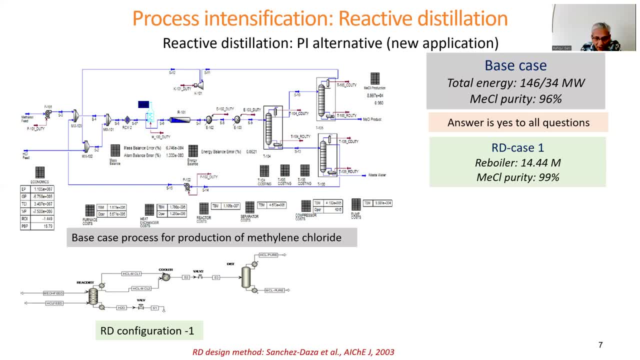 distillation column is much lower and the combined re-boiler duty of the two columns is much lower than the base column case. And we can replace the second distillation column with a membrane unit And also the combined re-boiler duty is much better And also the product purity is better. So we have 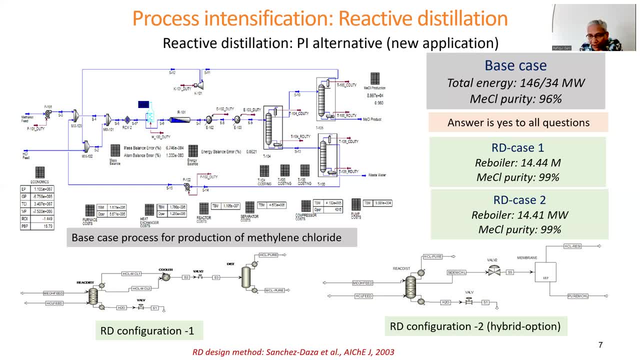 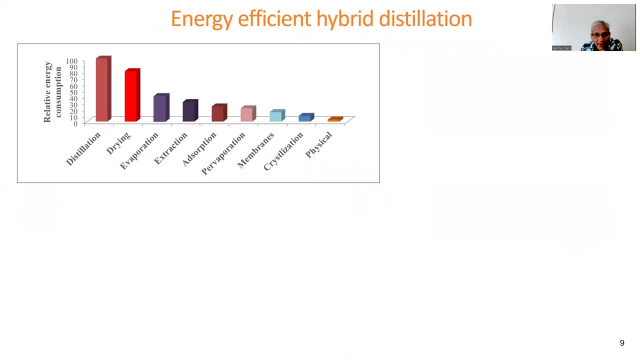 achieved significant improvement through intensification And we managed to find out very quickly for the given flow sheet whether the process intensification was possible. The second is hybrid. We know that chemical processes uses a lot of energy and distillation, as you can see in the figure, uses most of the energy. Now distillation is a very efficient technique. 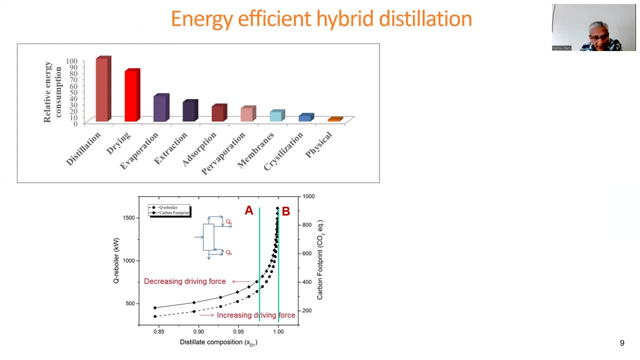 to separate, but until purity. And we can see that in that figure that cutoff point of purity is point A. Until that point A the distillation is very good, But in order to go from point A to point B it uses 80%. 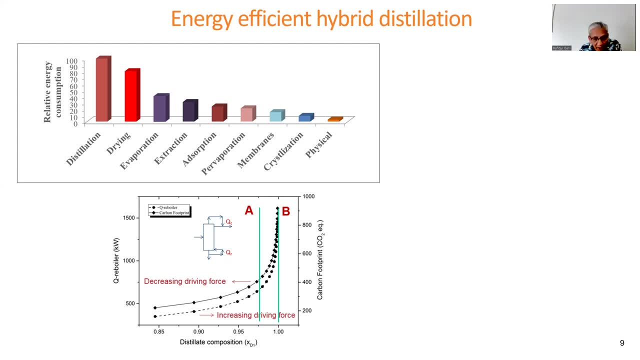 nearly 80% of the total energy required for that separation. So, then, the idea of the hybrid is: can we use distillation until point A and replace distillation from point A to B with something else that requires less energy, For example membrane? 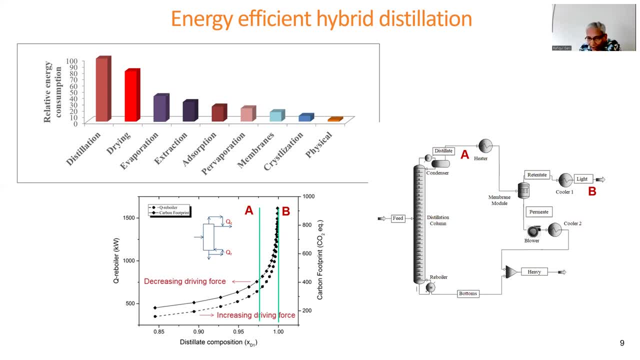 And this is the configuration. then for the hybrid We have the distillation of the distilled until point A, so the reboiler duty will be reduced, and then we put a membrane where the heavy boiling compound is, the permeate, so the flux for the membrane is reduced and we still get the same product purity that we wanted. 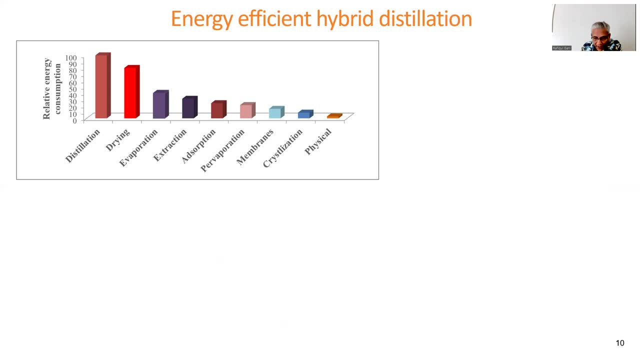 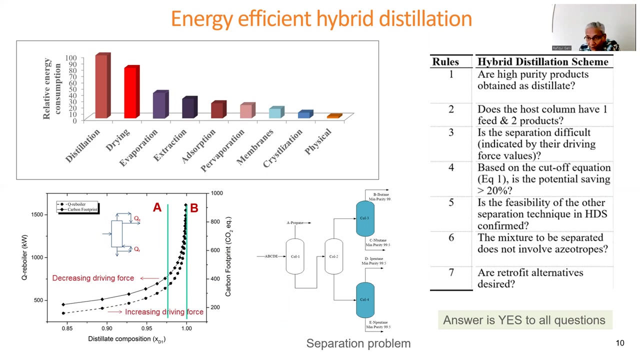 What is the consequence of this? Let us look at the design And let's take an example. Here is a separation process that can be found in many petrochemical refinery processes: separation of hydrocarbons. The two columns- shaded columns- use a lot of energy, so we can take any of those and we can answer the seven questions. Are high purity products obtained as distillate? Yes, 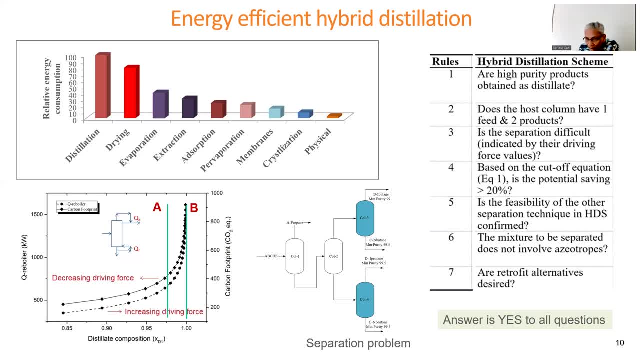 Does the host column have one feed and two products? Yes, Is the separation difficult? Yes, The more difficult, the more incentive to use a hybrid operation based on cutoff equation. is the potential saving? 20%? It can be easily seen from the figure that it would be. 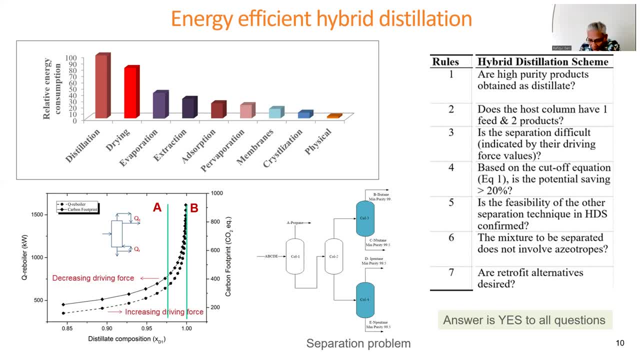 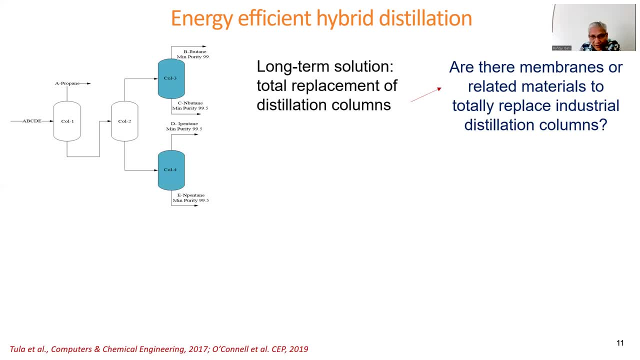 And the remaining questions are also yes. So if all these questions are yes, then we can convert this flow sheet and take each of these distillation columns, the shaded columns, into the short column. Yes, This is a short-term solution of hybrid scheme. We are not considering the long-term solution of totally replacing the distillation column, because those kind of membranes we need to find first. 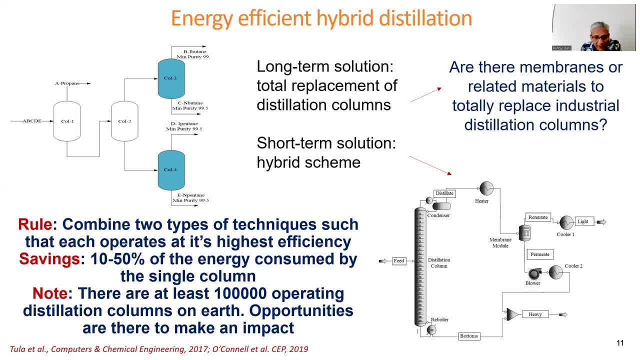 This is a win-win situation because we are combining two columns, two separation techniques at their highest efficiency. Savings of 10 to 50% can be achieved compared to the single column, Considering that there are at least 100,000 operating distillation columns on Earth. 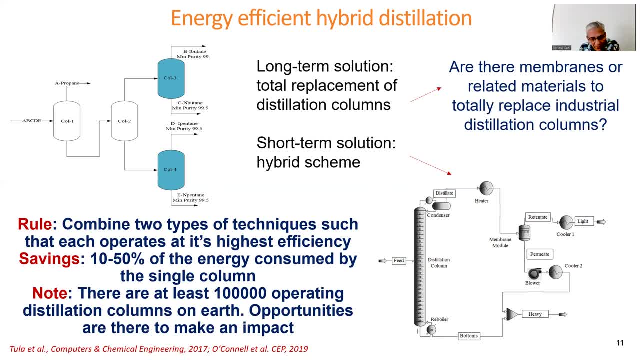 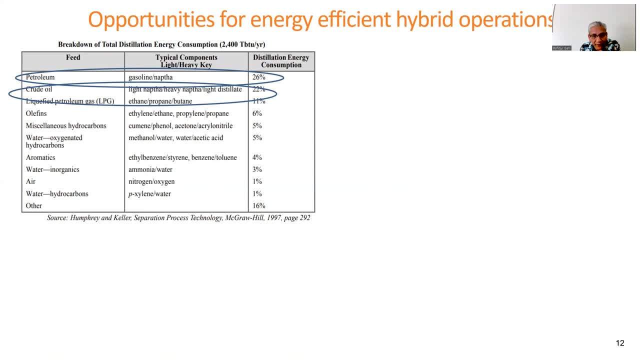 The scope and significance is very large, And this also can be seen from the fact that most of the energy-intensive distillation operations are using hydrocarbons And therefore, if we consider only the hydrocarbon separations, we can make a big impact in the energy savings. 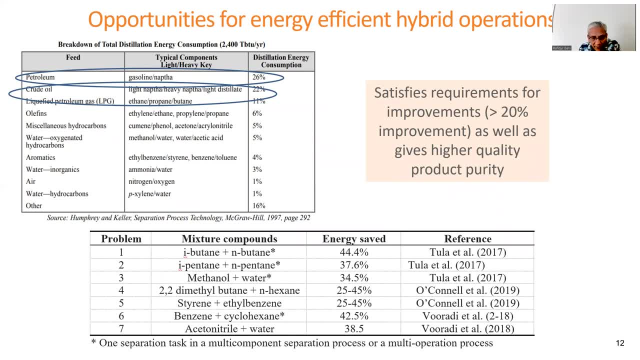 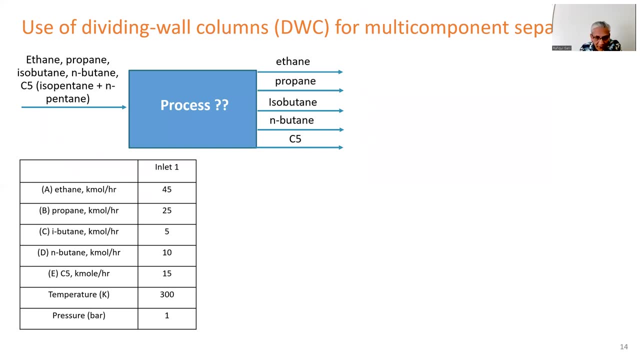 And here are some examples that we have already performed For which we have provided verified solutions. So the next one. we go to dividing wall column. We again have a process. because of confidentiality We cannot show the actual process, but it's separating of hydrocarbons. 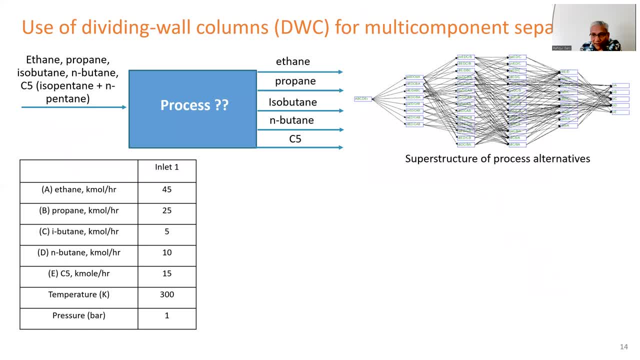 One feed giving five products. We can synthesize And the superstructure of all alternatives will give us 184 alternatives. But if we take only the distillation, that is the vapor-liquid separations, This is the sequence that is the optimal. 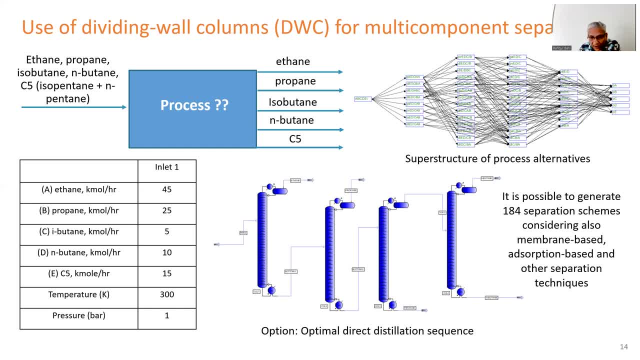 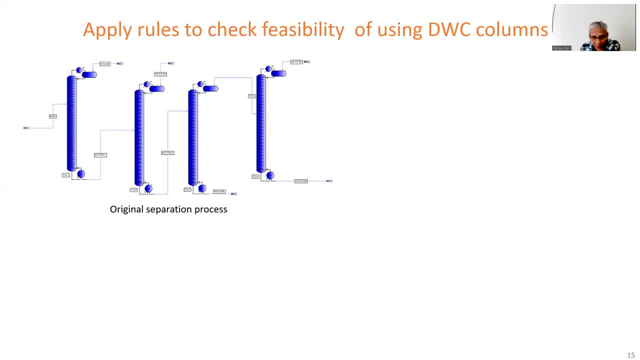 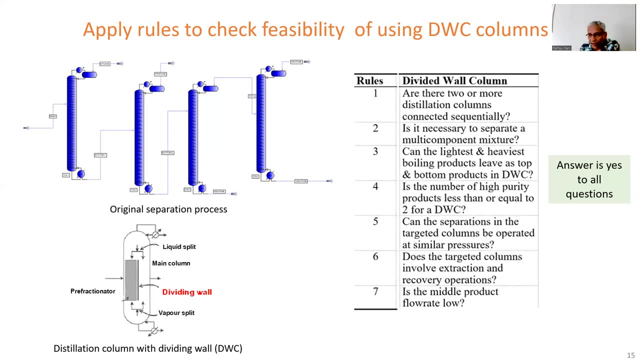 Now, on this optimal, we will try to see, using the rules, whether dividing wall column can be used to advantage. So here is the original process. We want to use a dividing column which looks like this. These are the questions And again, the answer to all these questions is yes. 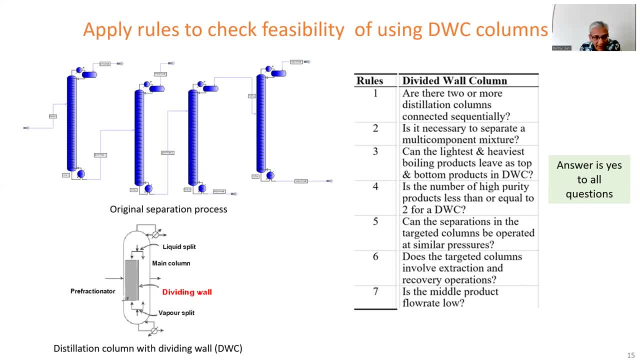 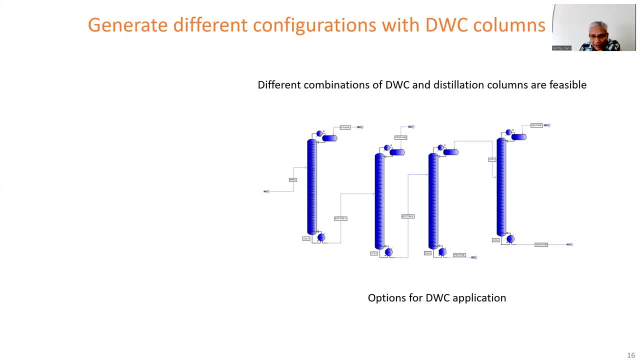 So we know that at least two of the adjacent columns can be replaced by this dividing wall column. So these are the again the four column flow sheet. The dividing wall column would be used for replacing two of them. The actual dividing wall column looks like the figure on the top left. 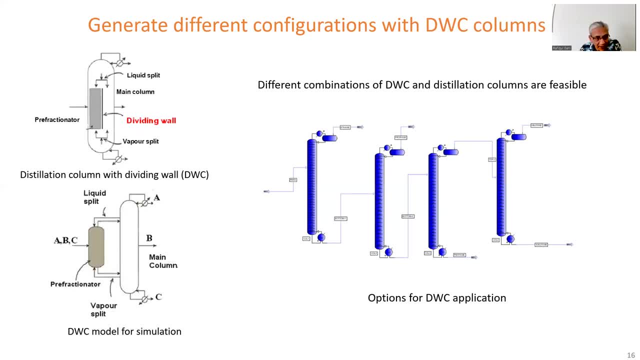 But for simulation purposes, the two dividing the two sections of the dividing wall column are arranged in a Petliou column configuration. So now, with this Petliou column configuration, we can see that we can take the two middle, We can take the two on the left. 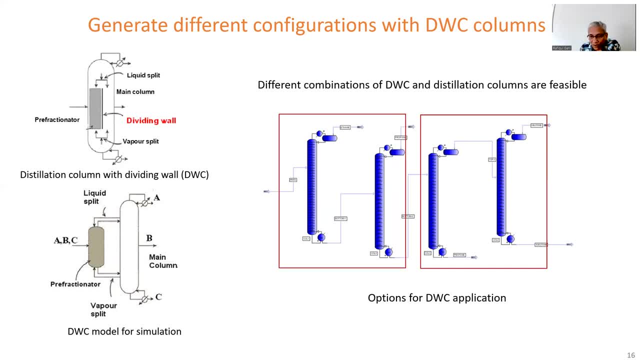 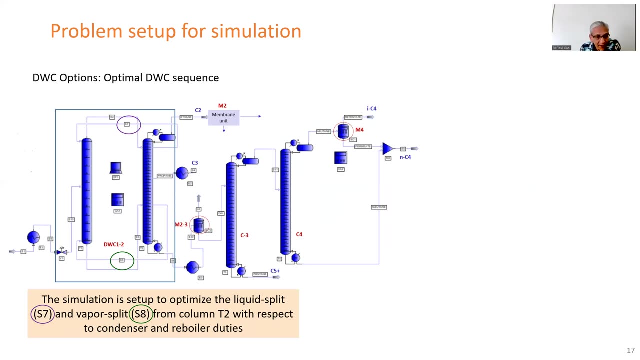 We can take two on the right Or we can take two dividing wall columns. So there are different alternatives. Which one is the best? We can enumerate and do the calculations. And the calculations also needs some calculations or verifications by simulation. Requires some extra notice to take. 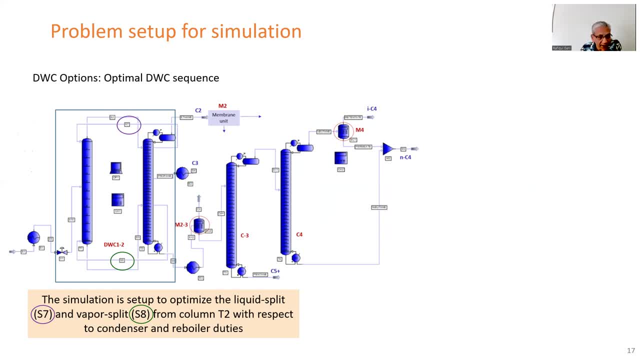 And this is that the streams S7 and S8, that is, the liquid from the top of the second column going to the first And the vapor from the bottom of the second column going to the first column. Those flow rates need to be carefully controlled in order to get the optimal solution. 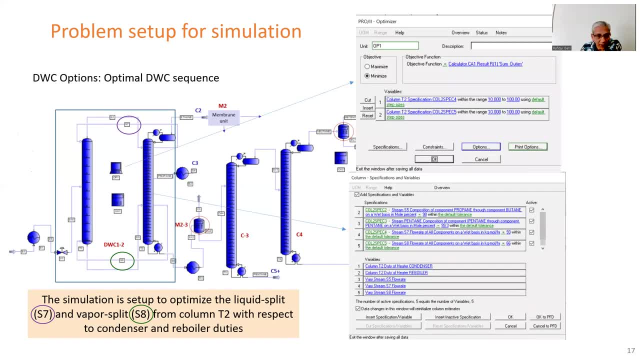 And so we configured the second column. We put a controller optimizer to control the flow rates connecting the second column with the first column, And if we have liquid and vapor flows with all the within, all the columns, then there should not be any problem. 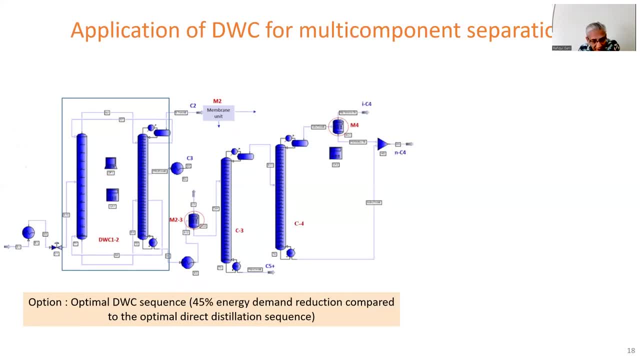 And then we find out that for This specific process the best configuration is to convert the first two columns into a dividing wall column. We get 45% energy demand reduction compared to the original. We can also add membrane units to further reduce the energy consumption. 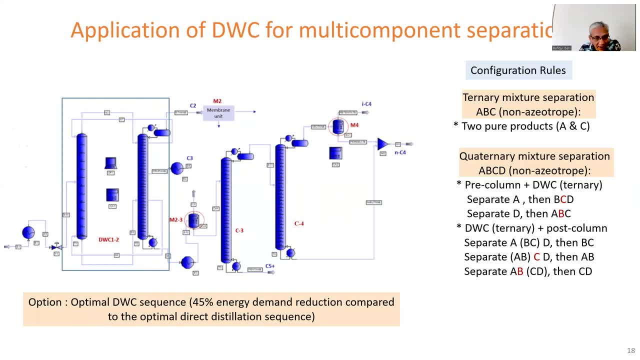 And then, based on the different configurations that we have studied, we have also put in rules, For example, if it's a ternary mixture, and ordering the compounds in terms of boiling point: lowest is A, next is B, next is C. 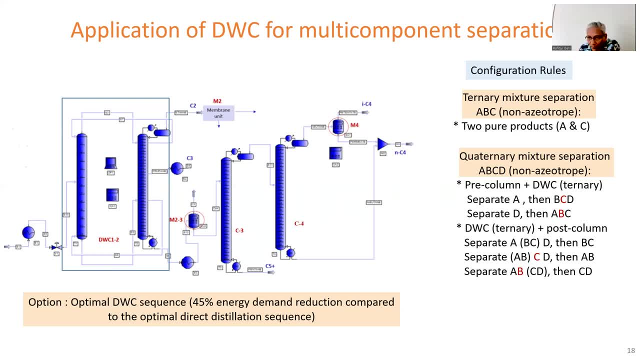 If we use a dividing wall column, compounds A and C can be pure products, but not B. If it is quaternary, there are different combinations possible If it is five component mixtures. we have created all kinds of rules to figure out which configurations would be the best.